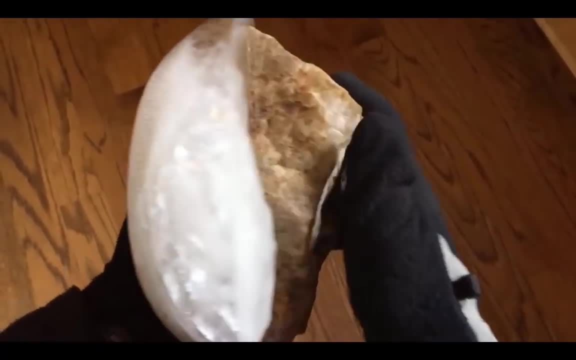 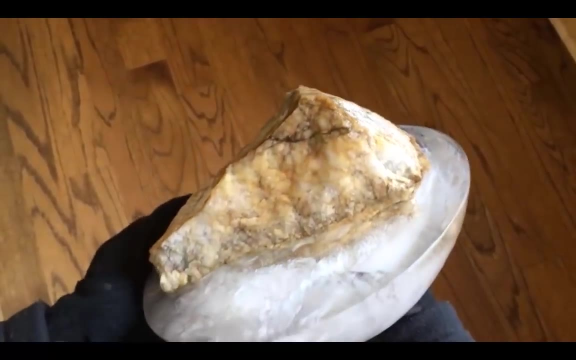 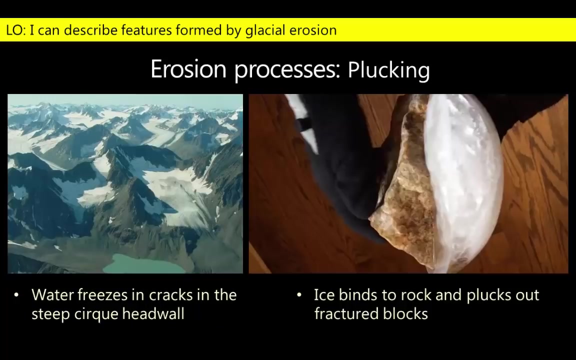 Who among us hasn't frozen a large rock into a block of ice to test how tightly the ice binds to the rock? When this happens in nature, it results in one type of glacial erosion known as plucking. Plucking happens when water invades cracks in the rock. As the water turns to ice, it binds onto the blocks of rock. 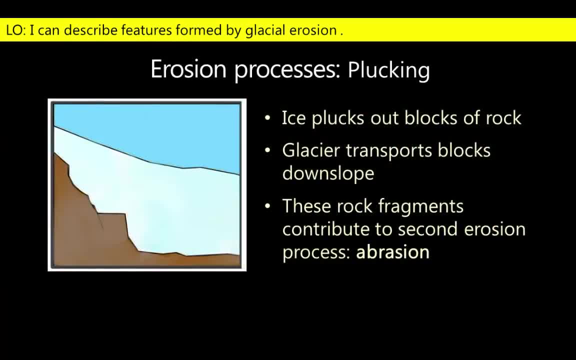 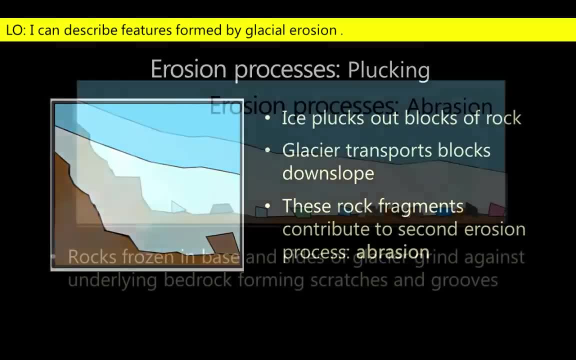 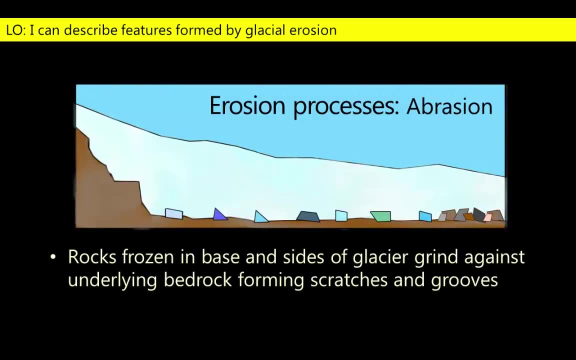 The motion of the glacier plucks the blocks of rock out of the cliff face, Embedding them in the moving mass of ice and transporting them downslope. Rocks frozen into the base and sides of the glacier act like sandpaper, scraping against the surrounding valley walls and floor in a second process of glacial erosion known as abrasion. 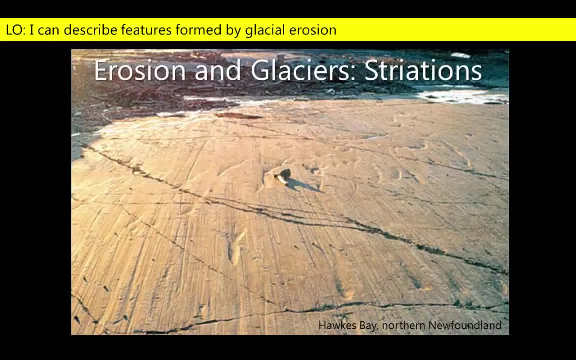 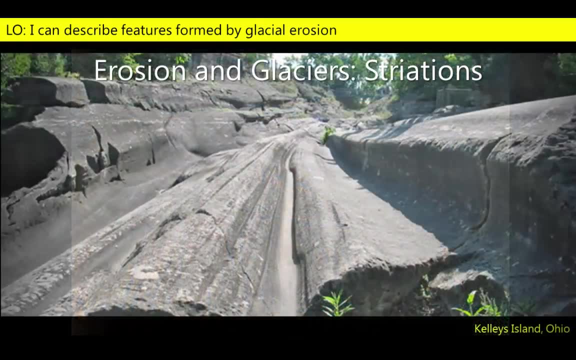 Abrasion leaves behind tell-tale striations in the bedrock that identify the direction of the motion of the ancient glaciers. Some striations, like these grooves, worn into this limestone bedrock, can be very dangerous, Indicating that they were formed below thick, powerful ice sheets. 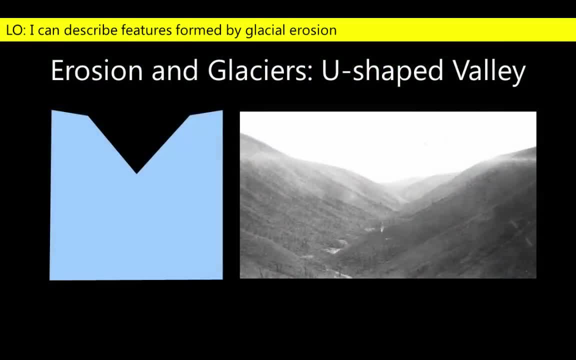 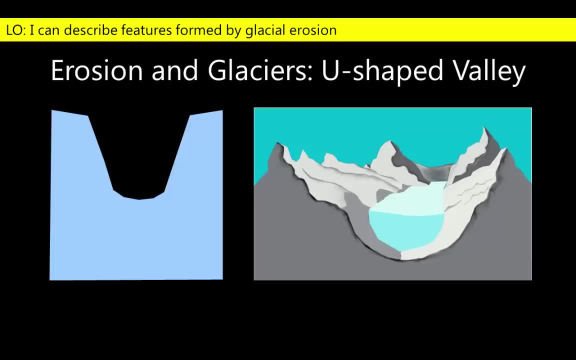 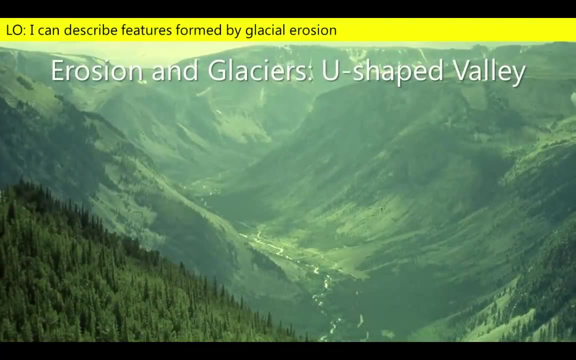 The combination of plucking and abrasion deepens and widens V-shaped stream valleys to produce a U-shaped profile characterized by a flat valley bottom and steep sides. Much like this example from Scotland And this U-shaped valley from the Beartooth Mountains in Montana. 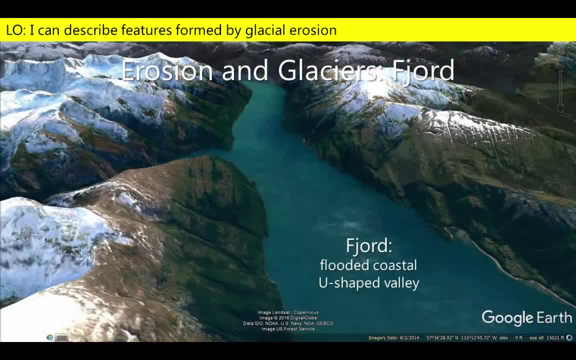 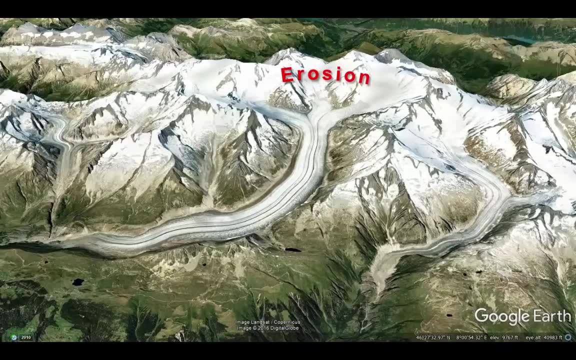 If rising sea levels were to flood one of these things, we would have to call it a fjord. If rising sea levels were to flood one of these things, we would have to call it a fjord. Up to now, we have been focusing on processes that cause erosion. 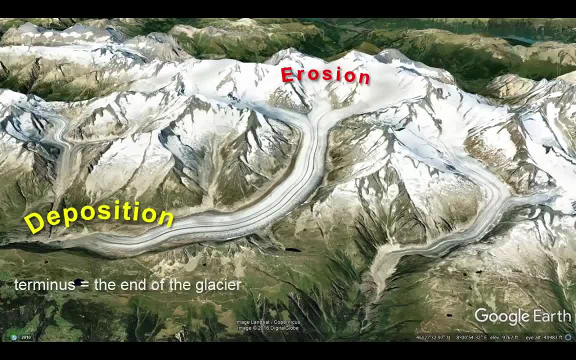 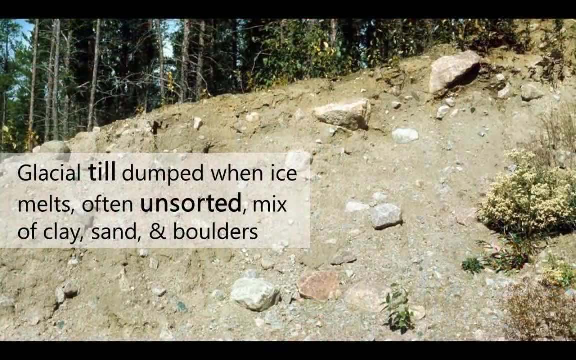 Now we want to turn our attention to features formed in glaciers' deposit material near their terminus. Most deposits left behind by glaciers are composed of a generally unsorted mixture of clay, silt, sand and boulders, known as glacial till. 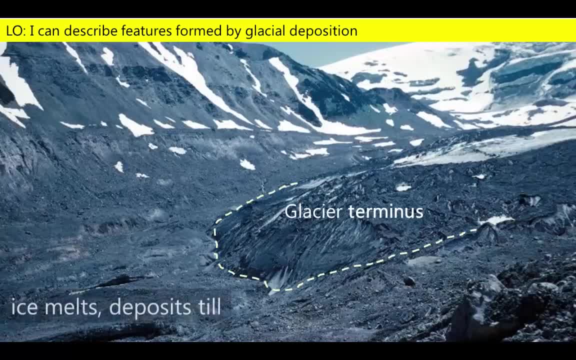 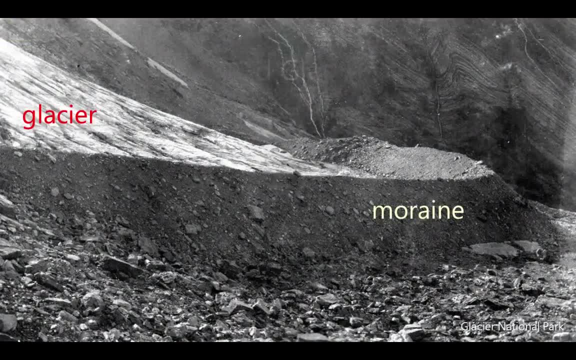 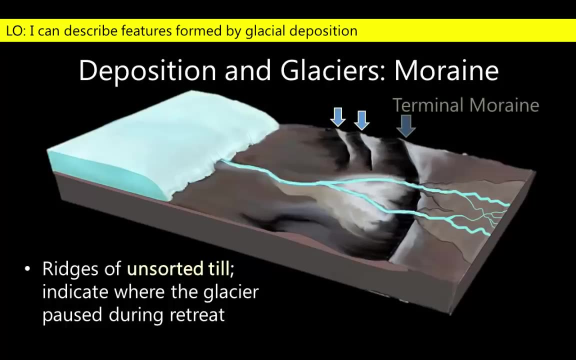 Ice that the terminus of a glacier will melt and dump piles of till. If the position of the terminus remains stationary for some time, it can leave behind a ridge of unsorted till known as moraine. Moraines essentially define where the glacier paused and the position of the moraine that is farthest down the valley. 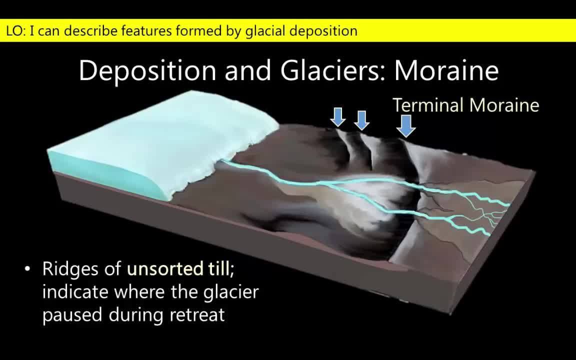 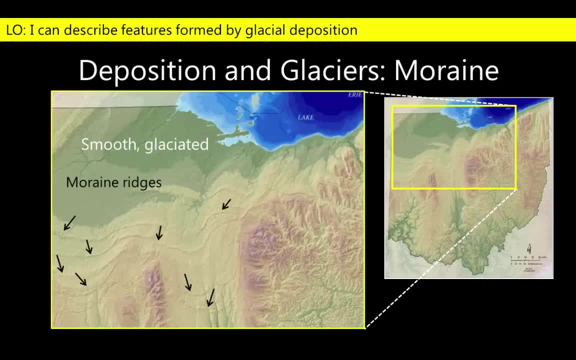 The terminal moraine indicates how far the glacier extended during its history. Ice sheets leave behind moraines that can be traced for hundreds of kilometers across multiple states. For example, this Shaded Relief Map of Ohio shows the positions of several moraines stretching across the glacier. 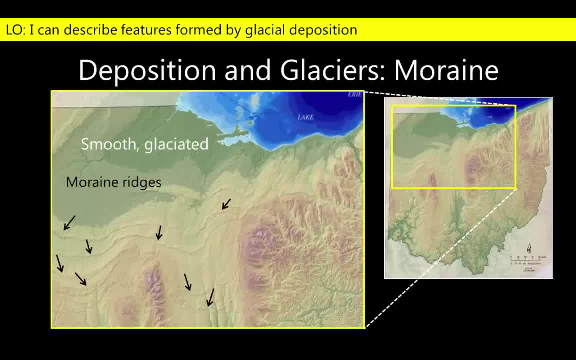 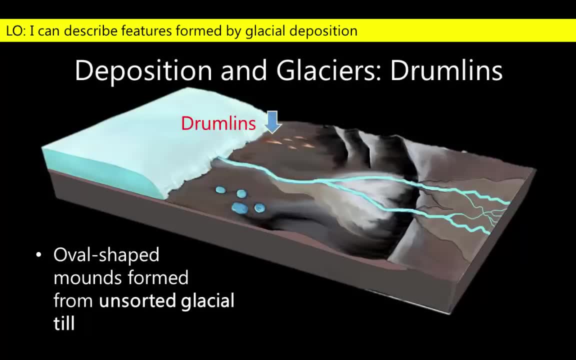 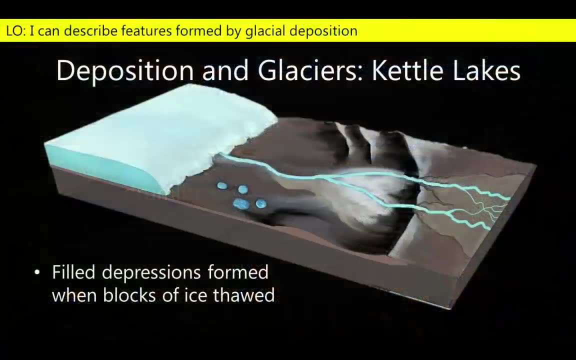 This is the northwest corner of a state and into neighboring Indiana. Piles of unsorted glacial till can be trapped by an advancing glacier and shaped into oblong mounds known as drumlins that narrow in the direction of glacial motion. Behind the moraines we also find hundreds of small lakes, known as kettle lakes. 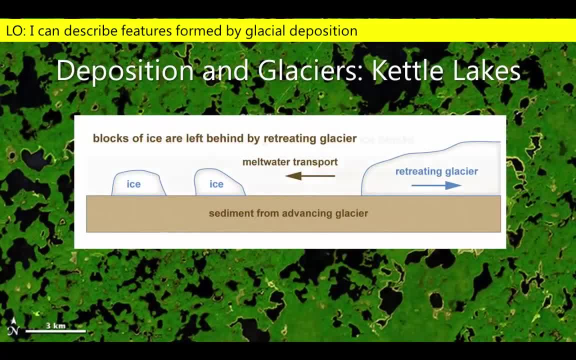 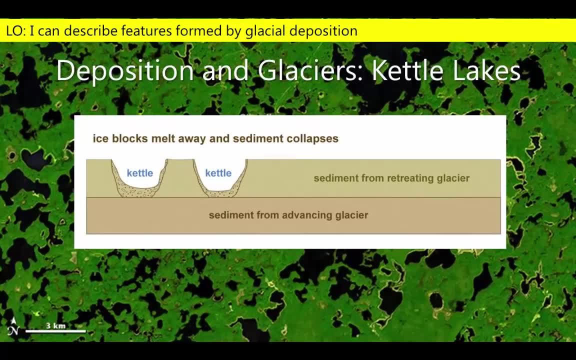 Kettle lakes form when blocks of ice break off or retreat in glacier and are subsequently buried. The ice will continue to grow, gradually, melts, forming a depression in the glacial sediment known as a kettle. These low areas may then be partially filled to form a lake, just like these kettle lakes. 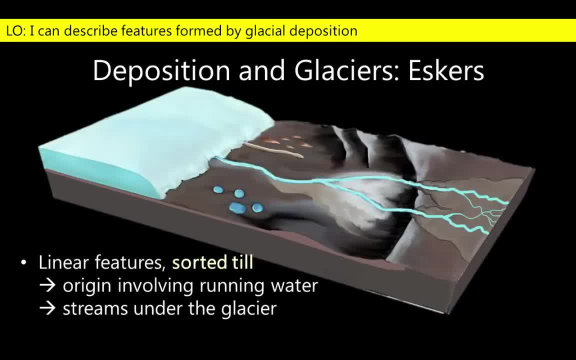 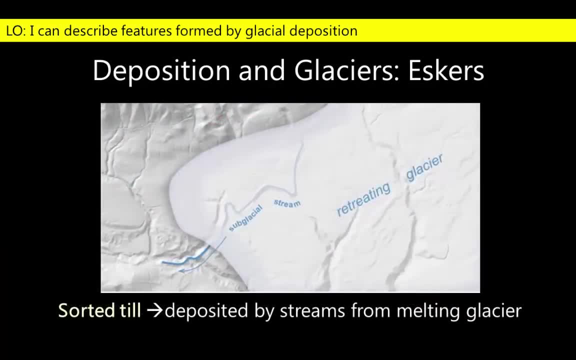 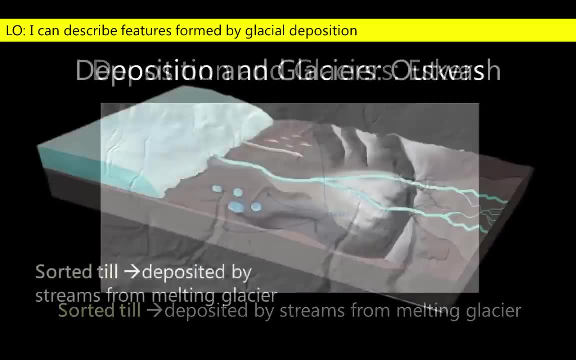 in North Dakota, A feature known as an esker may be formed when till is sorted by streams flowing at the base of the melting glacier. The sediment deposited within these subglacial streams leaves behind a skinny, sinuous land form. Likewise, as the glacier melts and its ice turns to water, meltwater streams, transport. 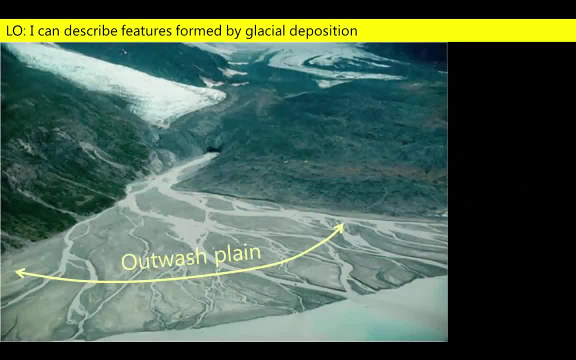 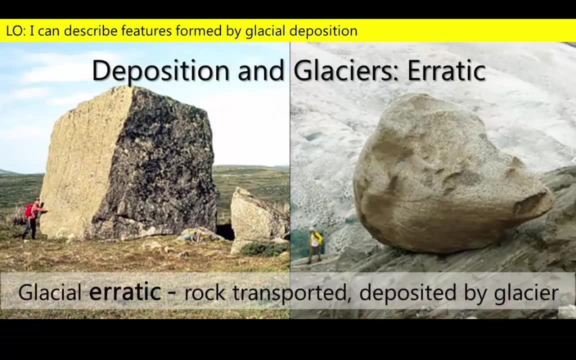 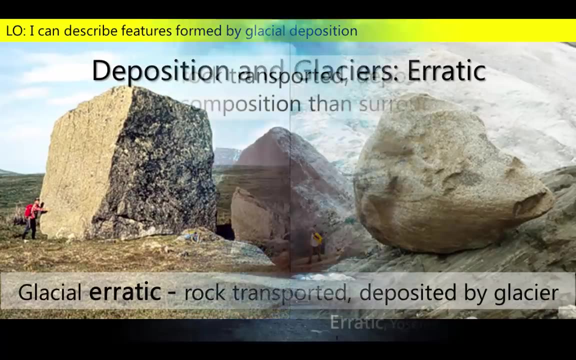 sediment away, depositing some of it in the adjacent outwash plain. Thick ice sheets can pick up very large rocks known as erratics from one location and deposit them elsewhere, sometimes hundreds of kilometers from their source. By matching the geology of the erratic with their source area, we can unravel the direction. 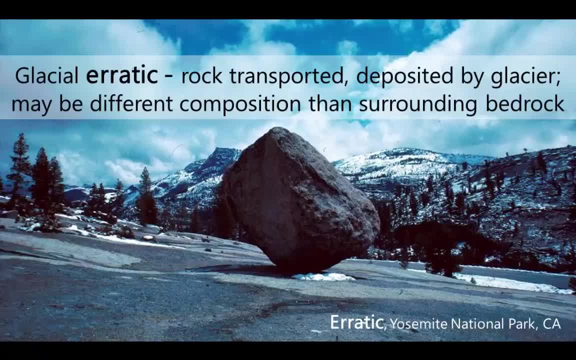 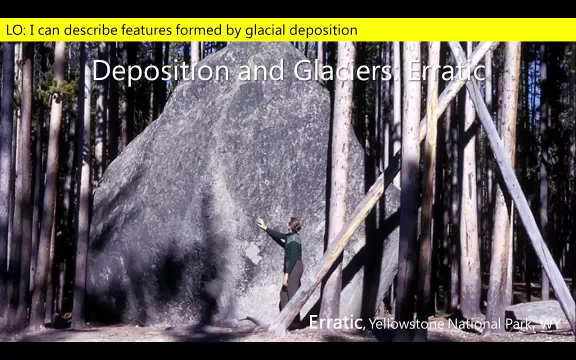 and distance of motion of the ice that makes the ice melt And that brings us back to our 500-ton friend among the trees in Yellowstone National Park. This boulder of metamorphic gneiss sits on top of volcanic rocks, hundreds of millions. 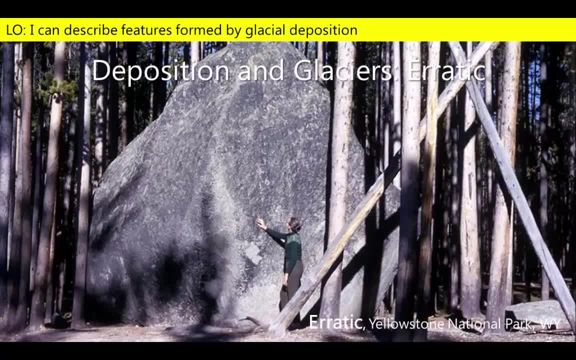 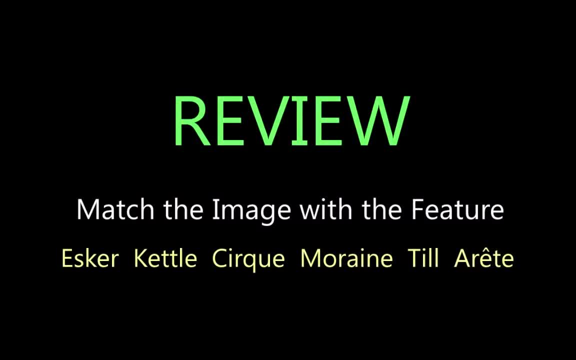 of years younger in age, And the boulder must have been carried at least 25 kilometers from its source. Let's finish off with a matching exercise. We will show you pictures of four glacial features. Match each one with a term from the previous slide. Let's start with a matching exercise. We will show you pictures of four glacial features. Match each one with a term from the previous slide. Let's start with a matching exercise. We will show you pictures of four glacial features. We will check your answers when you are done.